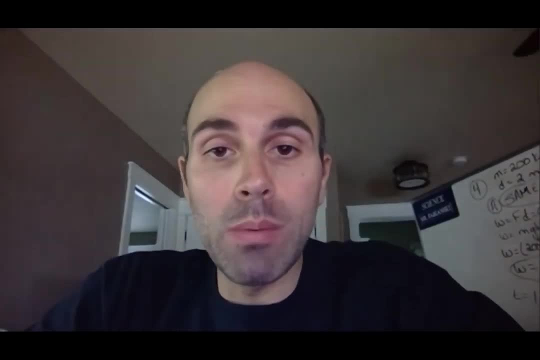 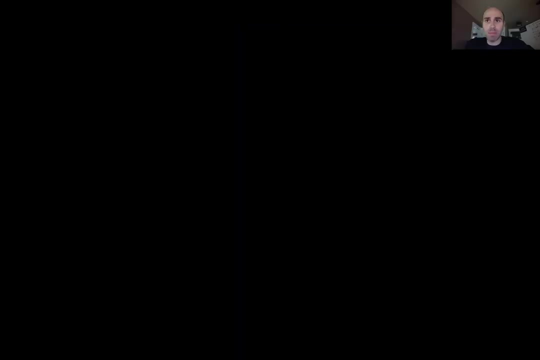 Hello and welcome everybody. Today we will be wrapping up our PowerPoint on plate tectonics by looking at the different types of interactions between the continental and oceanic plates. So, without further ado, let me bring up the old PowerPoint and explain to you exactly what we are. 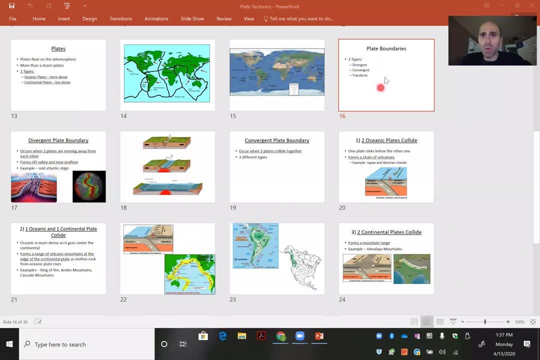 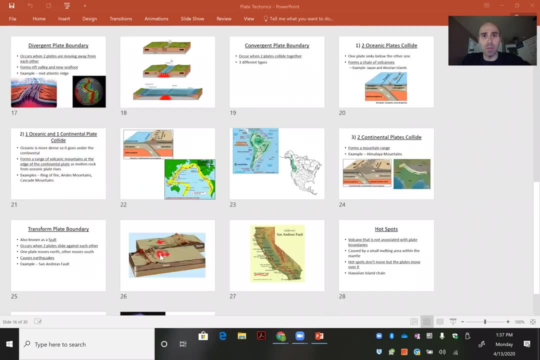 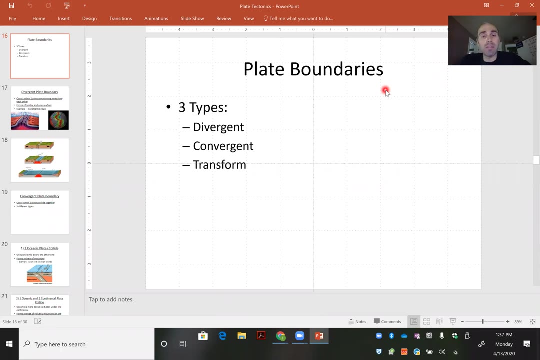 going to be doing today, Excuse me. So we are going to go from slide 16, talking about the different types of plates, all the way down to the very end. So excited to start this with you guys today. So let's dive on in. So, plate boundaries: There are three different types. 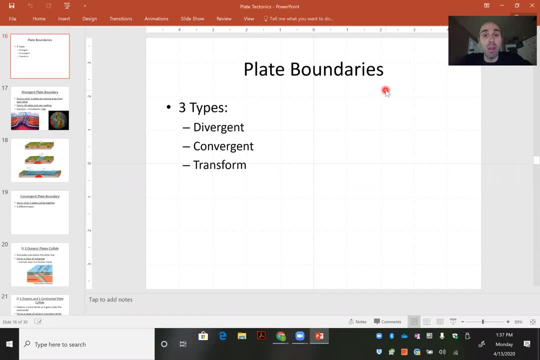 of plate boundaries that you should concern yourself with. We have divergent, convergent and transform plate boundaries. Divergent means the plates are moving apart, Convergent means they are coming together, And transform means they are slip, sliding past one another. Okay, 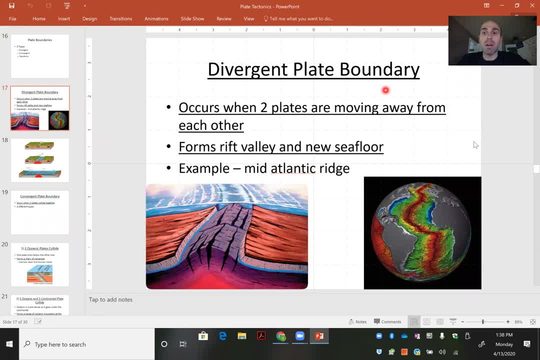 Three different types. Now a divergent plate boundary is pretty simple. There's only one subcategory. It occurs when two plates. they could be oceanic, they could be continental crust, they could be a mix of the two, meaning a continental and an oceanic, or two oceanics. 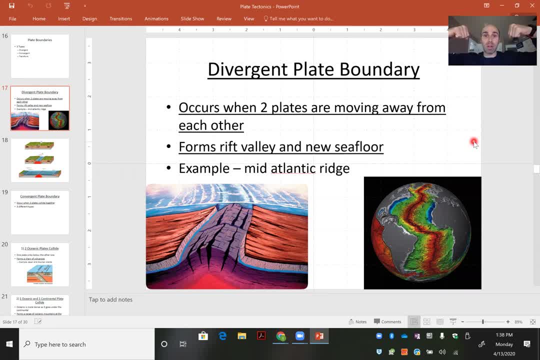 or two continentals. It occurs when they move away from one another. Okay, They are moving away, They are opening up. A crack is forming. It's opening up Right now. it's closing up. It's moving up in the earth, And that is what a divergent. 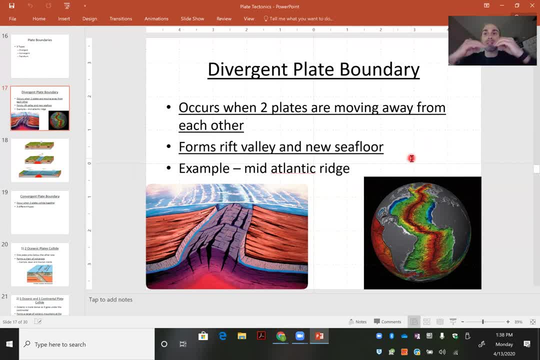 plate boundary looks like This plate boundary forms a rift valley near the sea floor, meaning that has it opens up. It has these two peaks that form. Okay, So these two peaks form on either side and you get a valley in the center. So you can see, right here we have this. this. 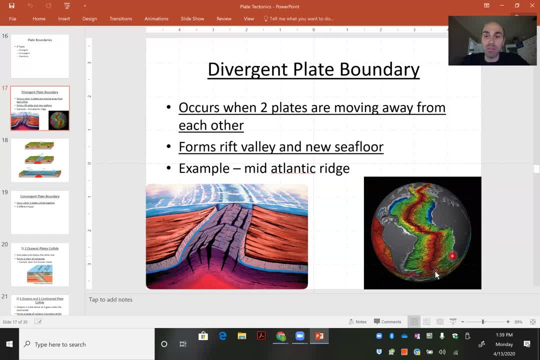 rift valley. we have two peaks and the valley in the center or the mid-atlantic ridge, and if you look, here is north america, south america, africa. this is the atlantic ocean, right here, looking through there, you see this red giant seam. that is the 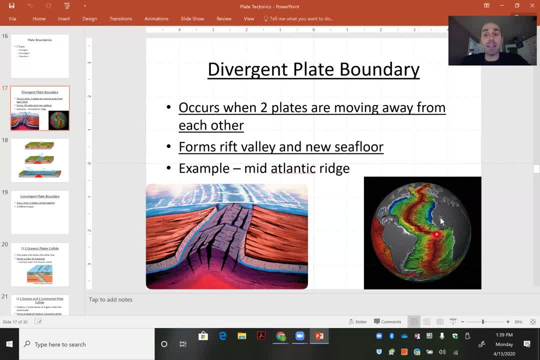 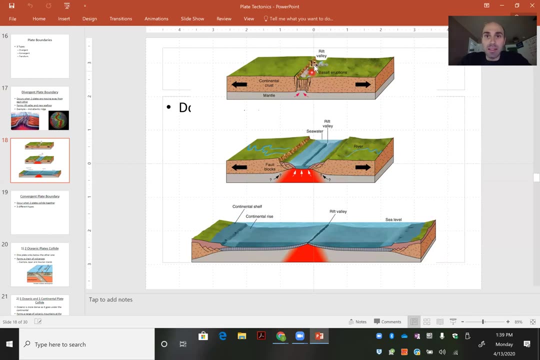 mid-atlantic ridge, the mid-oceanic ridge, and that is due to the divergent plate boundaries moving apart on either side. they are going in opposite directions. okay, so a divergent plate boundary, they move apart here. you can see, this is a wonderful example of a valley occurring here. 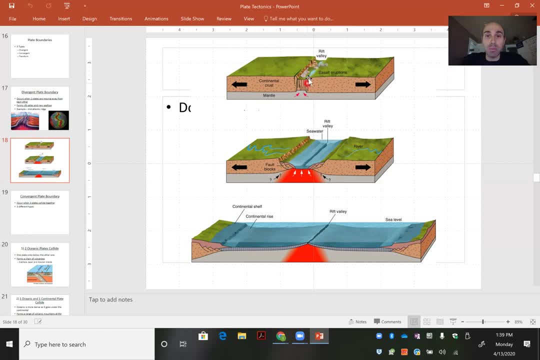 we see that as the two plates move apart, you create a rift valley. uh hot, magma moves up, creates new land. there's that rift valley right there. this is showing how you actually get a sea that forms. originally, when we had pangea and everything was close. 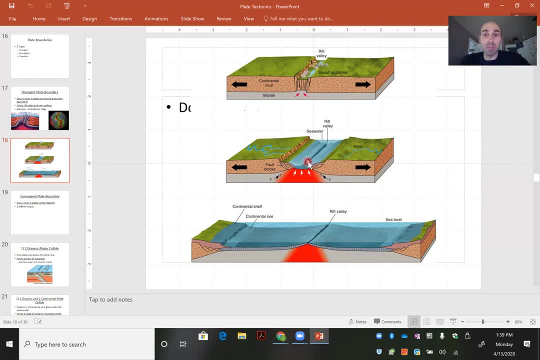 all the continents were close together. they opened up as they opened up throughout the millions of years. you get the formation of the rift valley and the two plates move apart and they are moving apart. they move apart here. you can see, this is a wonderful example of a valley occurring here. 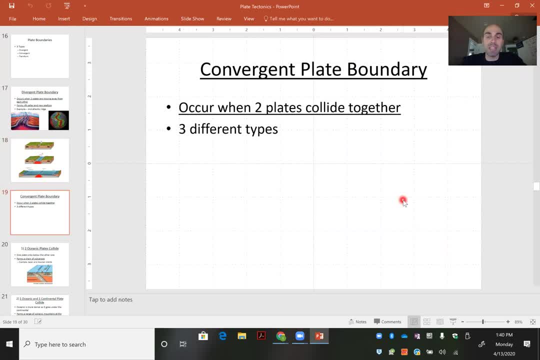 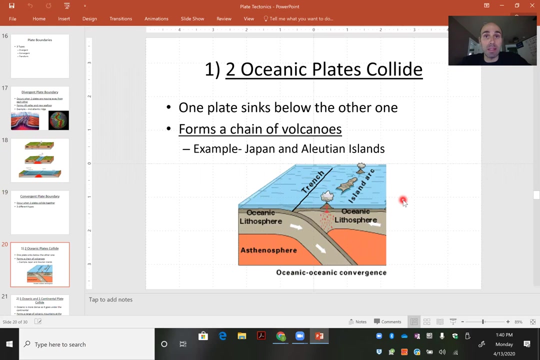 of a- C. the next type of boundary is a convergent plate boundary. so we had a divergent where they are moving apart. now we have a convergent where they are coming together. of this convergent plate boundary there are three different subcategories. okay, the first type would be when two oceanic plates collide. 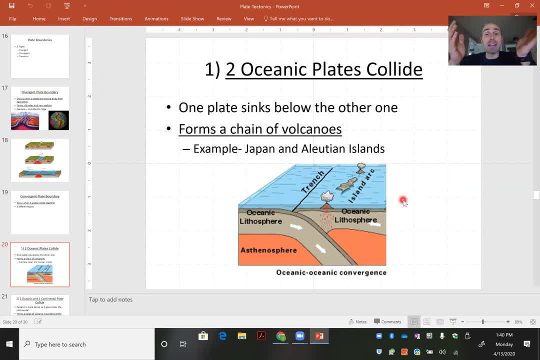 remember, we have oceanic plates and we have continental plates, oceanic crust and continental crust. in this case, it's when two oceanic plates comply, come, collide. now, oceanic plates are thinner but more dense than continental plates. so when two oceanic plates collide, one plate will sink below the other. it forms. 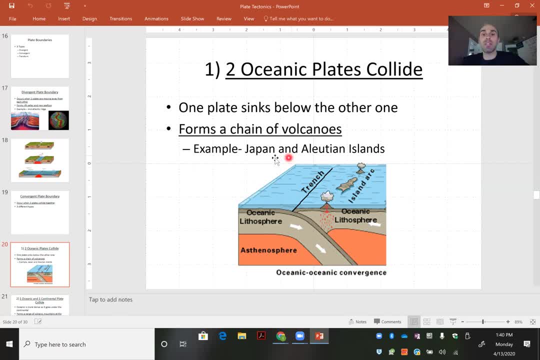 what's called a subduction zone. an example of this would be a Japan and the Aleutian Islands. we see that as it slip, slides underneath the other one, one gets pushed up here and that's where you get volcano and your islands, the Aleutian Islands, and a. 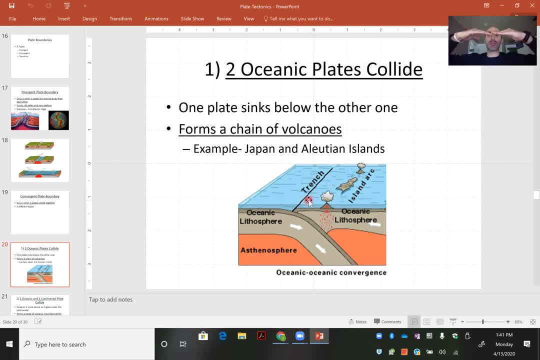 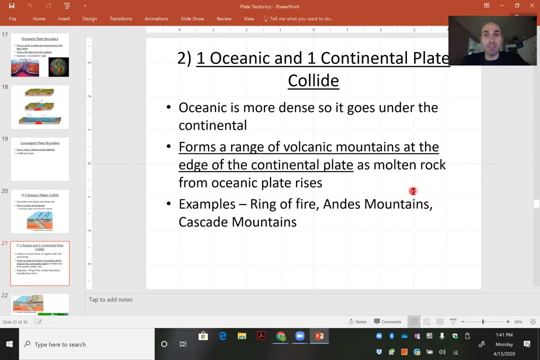 trench is completed because, think about this- as they're coming together, you start to get one sliding under, right there, in that area, right here, this area, you get a trench that forms okay. so a trench is completed with the formation of an island chain. the second type is when you have an ocean plate and a continental plate colliding. so now you 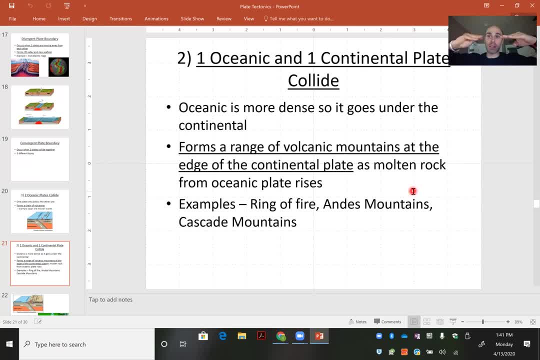 have a thin ocean plate in a very large continental plate- right, this huge, it's very big continental plate- and they're gonna combine here. what do you think would happen? you're correct. I'm assuming that the thinner plate would slide underneath the thicker plate in the ocean plate would slide underneath the 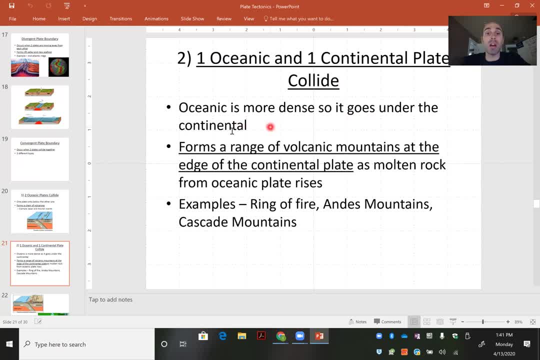 continental plate. the ocean plate is more dense, so it goes under the continental plate. it forms a range of volcanic mountains. 올 때, 올 contesto. continental crust, and you also get a trench worthy to meet. okay. examples of this would be the ring of fire, the Andes Mountains, the Cascade Mountains. here's a. 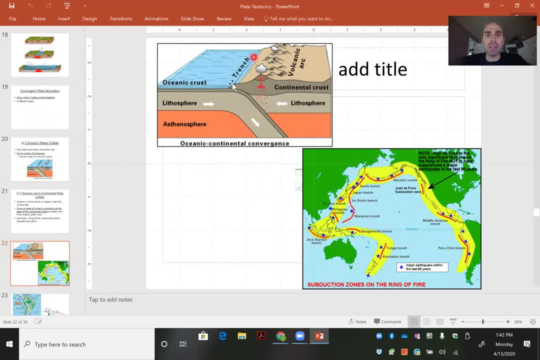 little diagram you can see the trench is also formed right here. you can see the formation of these mountains. this is due because the crust is coming down, it's being reheated and then rising to the surface again. this here is the ring of fire. this is formed by the convergence of the oceanic plate on to the 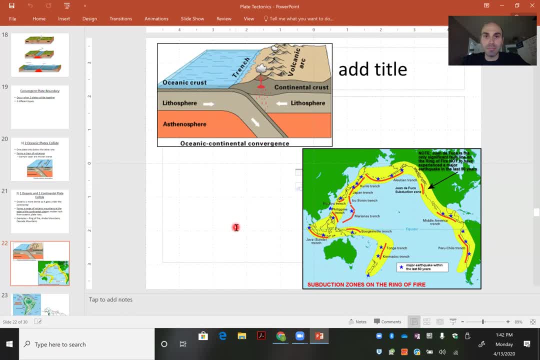 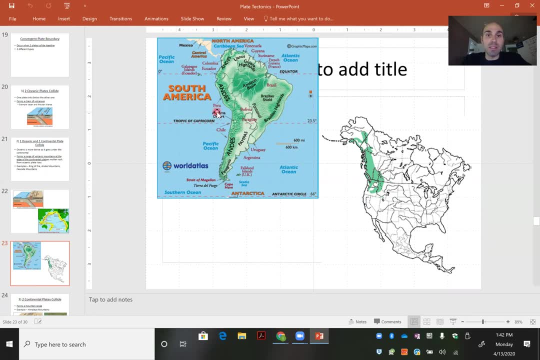 continental plates. again, here we go. the Andes Mountains are formed from the South American plate moving in this way, and the continental plate moving towards it. again, they're combining. you get the formation of these mountain ranges along the entire coast of South America, along Chile, and you get the 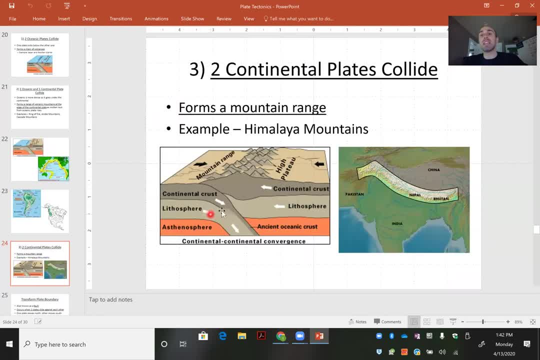 formation of the Andes Mountains, along Chile, along Honduras, and you get the of a trench here. The third type is when two continental plates collide. So we had two oceanics, we had an oceanic and a continental, and now we have two continentals. Here you get. 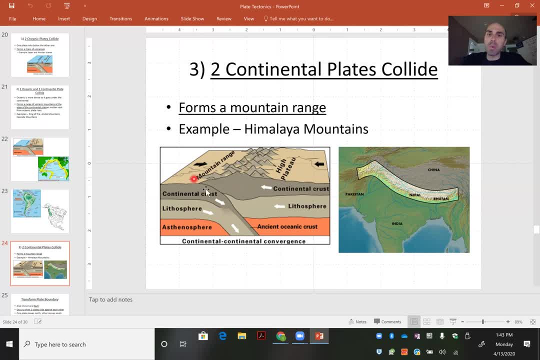 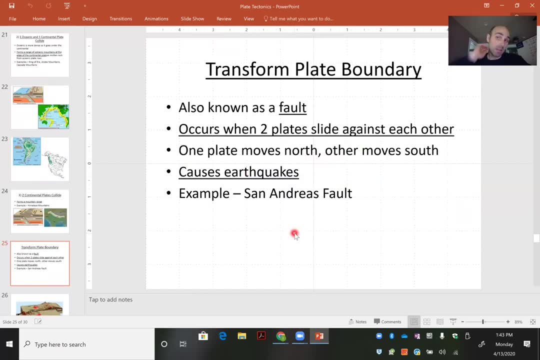 pretty much the same idea. You get a mountain range that forms with little to no trench. Himalayan mountains would be an example of this. So we've talked about convergent plate boundaries. We've talked about divergent plate boundaries. Now, what we will talk about is the transform. 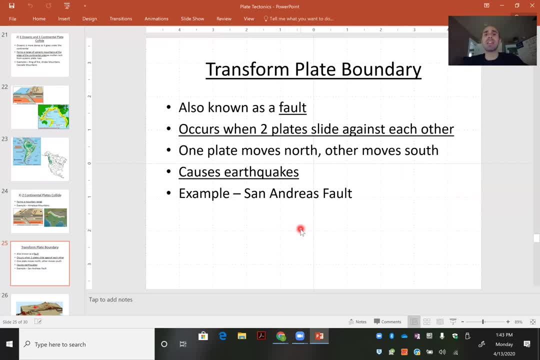 plate boundary. Transform plate boundary is where they slip, slide past one another. You would know this as the San Andreas Fault right. What occurs at San Andreas Fault Watch? You're right, earthquakes. Earthquakes are major, major indicators of transform plate. 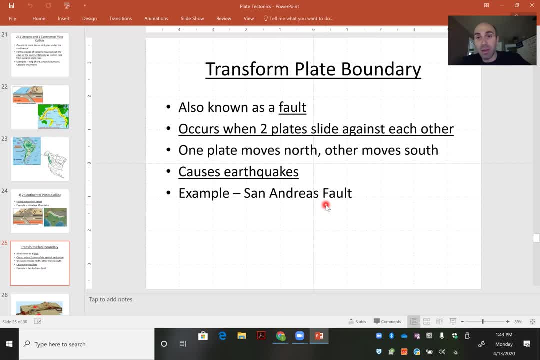 boundaries. One plate will move north, one plate will move south. They are slip sliding past one another. As they slip slide past, there is so much friction that, as they break apart, it's releasing this friction, this vibration, this cracking of rock, this fracturing, and that is what creates your 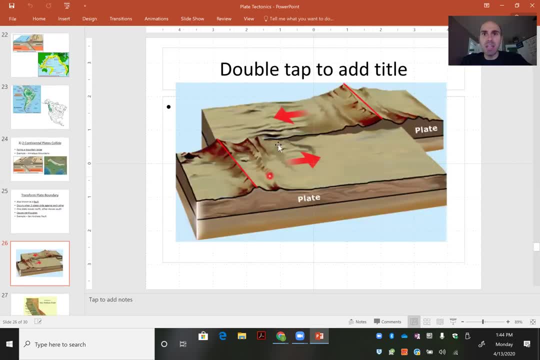 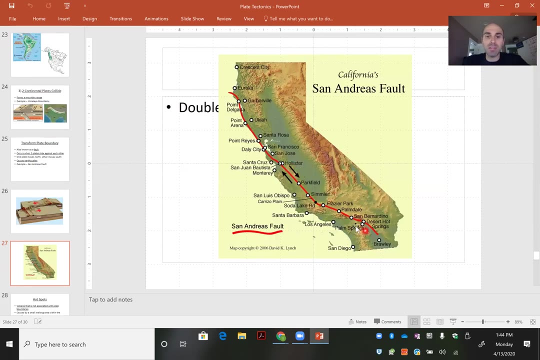 earthquakes. You can see here. these two mountain ranges used to line up together, but we have one plate moving south, One plate moving north and they are creating a transform plate boundary, The San Andreas Fault. we could see the majority of California is moving down, while southern 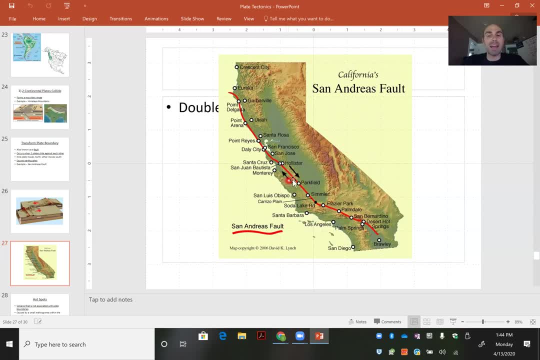 California and western California is moving up. It's not that it's going to fall into the ocean, It is just relocating and moving up. We see, along this boundary there is a large fracture zone and as it fractures, with every slight move it releases vibrations, and those vibrations are 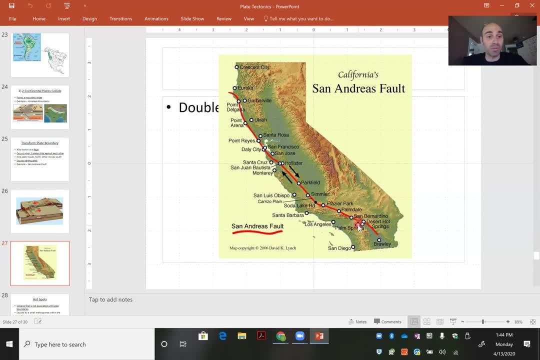 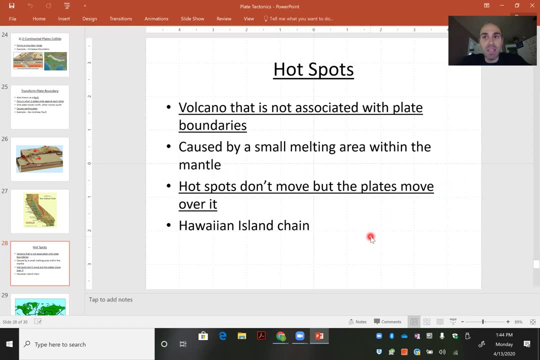 felt as earthquakes. We're almost there, guys. just three more slides Now. hot spots are not a plate boundary. however, volcanoes are associated with plate boundaries and these are caused by small melting areas within the mantle. Hot spots do not move, however, the plate moves above it. 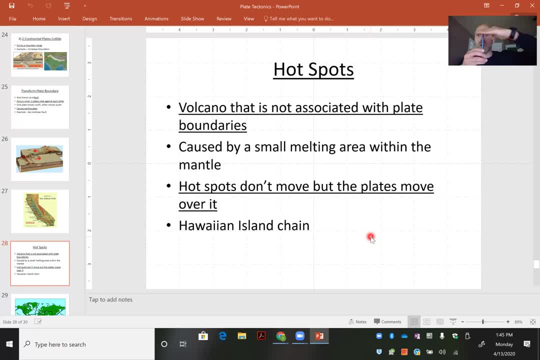 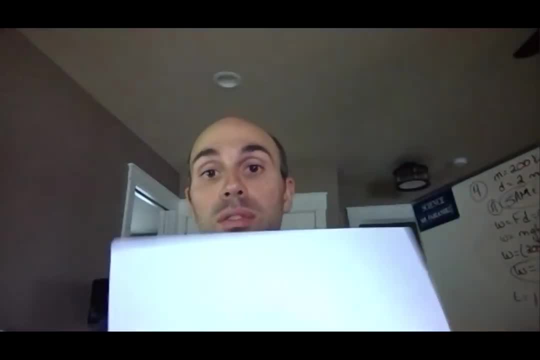 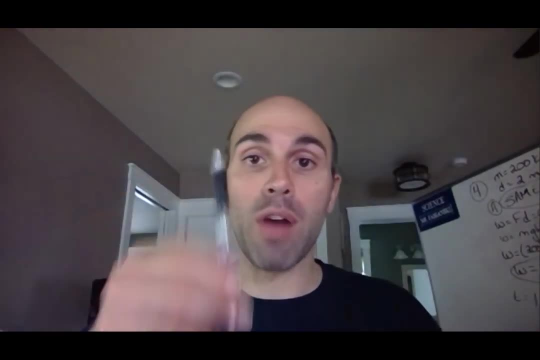 So if this were to be your hot spot as you are moving over it, actually let me show you, guys with a piece of paper here- and I'm going to take off screen share so it's easier to see- This is our plate. It's a movable plate, that's a piece of paper, but that's our plate and here we have our 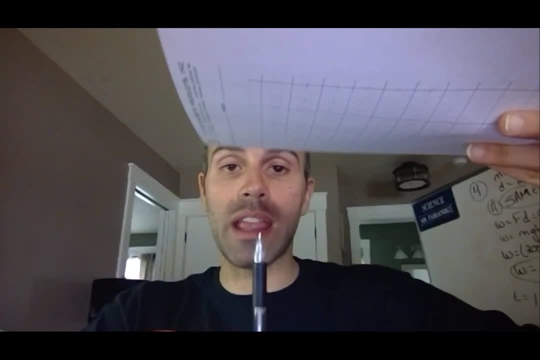 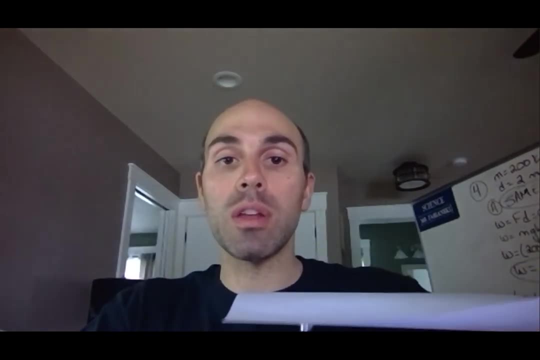 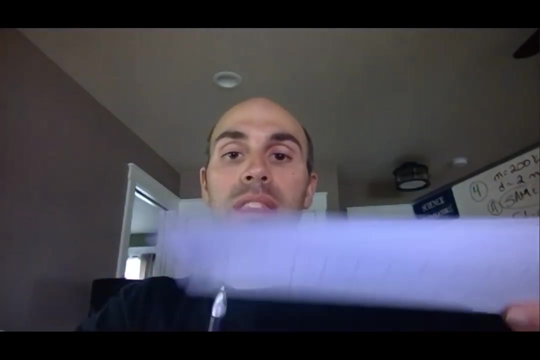 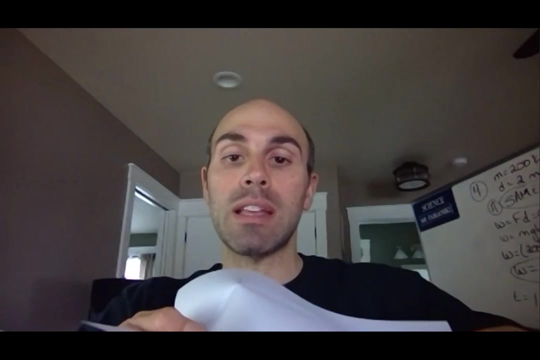 hot spot. So the hot spot will say it's still right in the center of the screen, but as the plate moves over, right as that plate moves over, you can see the hot spot. originally will start here, but then as the plate moves over, the hot spot will start and poke through there and then as it moves over again it'll. 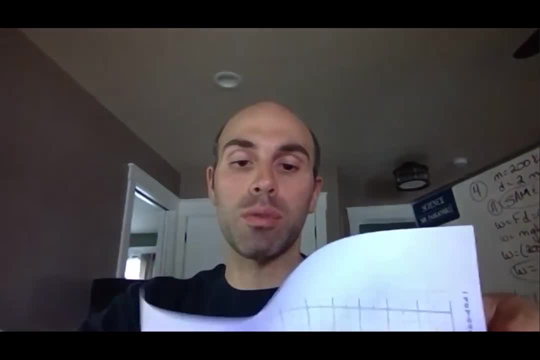 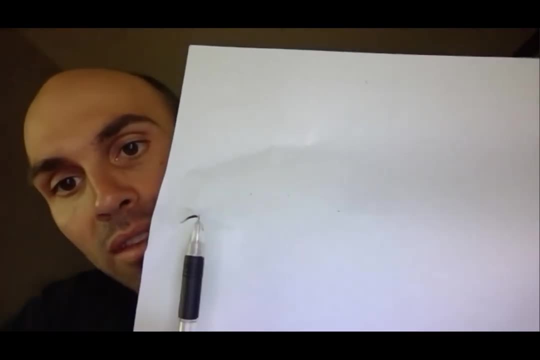 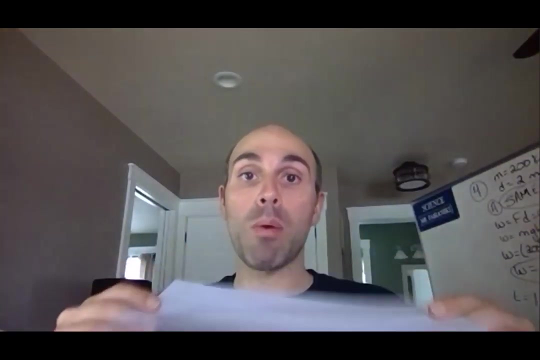 poke through there. As the plate continues to move, it will poke through again. This really would be better in person, but you can see. what you actually get is the movement of this hot spot from here to there, to there to there and so on. So the plate moves, but what you get is the hot spot.